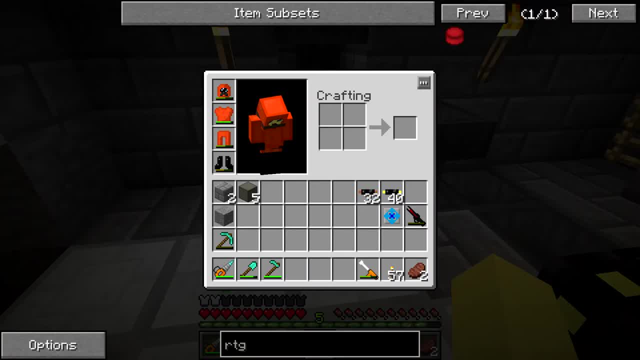 So unfortunately I can't click on this thing. but if we go and look at the radio it should be enough to just type in radio. so if we look at these they say the power output is 1 to 32 for heat units or EU per tick. 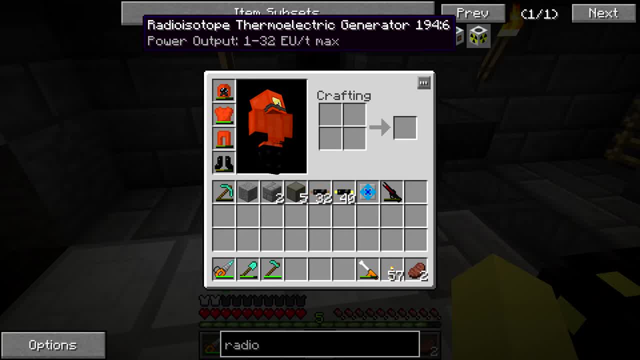 Well, that doesn't seem that bad if you think about it, but actually it starts at 2 and goes to 64 EU per tick, So it's a little deceptive when you're looking at the tooltips in NEI, because you can't get a lot of power generation from it. 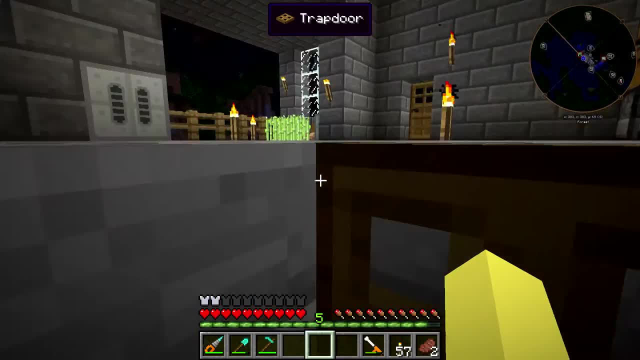 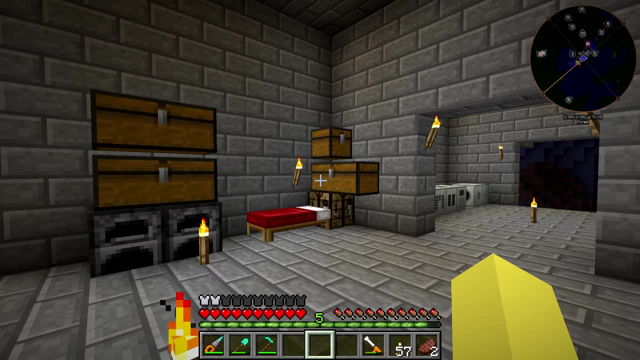 So I decided that, instead of making something that could potentially blow up my base, I'm going to make something that might use radioactive material and get us good power, but it won't have the threat of blowing up and I don't have to maintain it at all. 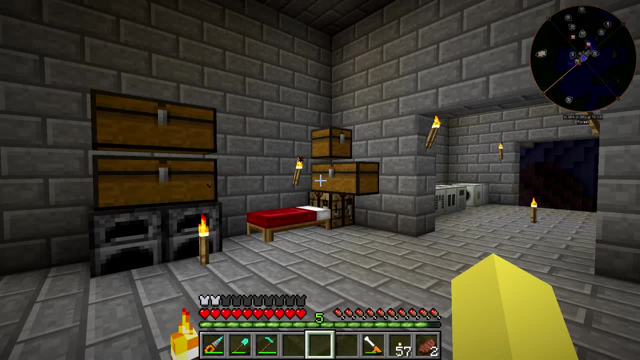 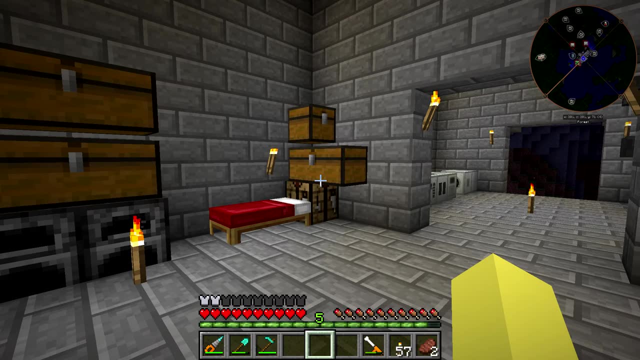 So the reason that this is great for me is because I at least have three nuclear reactors, three different kinds of nuclear reactors, all running at the same time getting power, or steam to get power. so I do have a lot of uranium fuel rods, specifically. 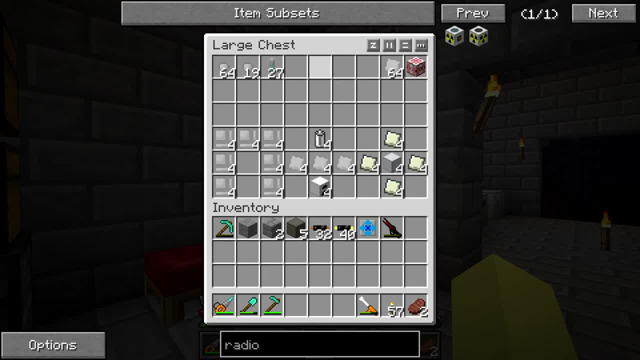 that I can turn into plutonium and then we can make RTG pellets from it. So my goal today is to make- I have the stuff to make- four of these radioisotope thermoelectric generators, which will eventually be running at 64 EU per tick each. 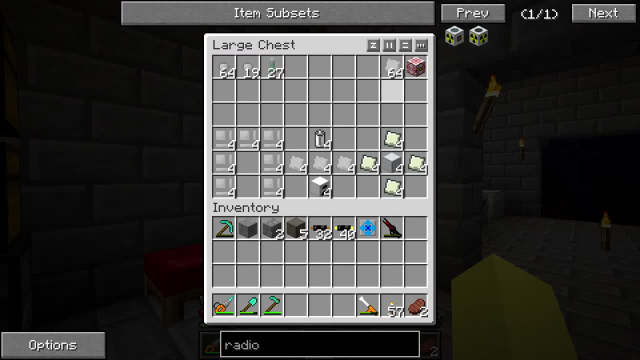 and essentially the goal is to just fill them up as much as I can progressively. This is a full batch of the depleted uranium cells from the plutonium generating nuclear reactor that I have downstairs right now. I do have a little bit of plutonium just here and there from extra fuel rods. 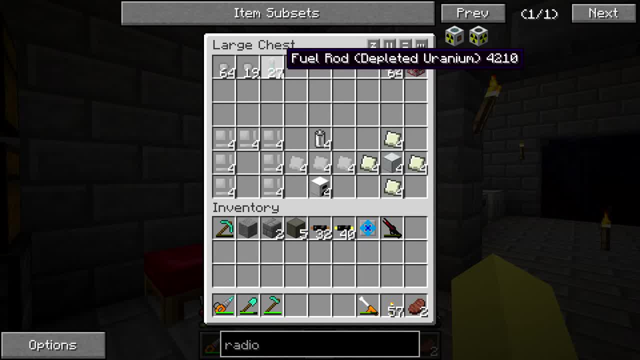 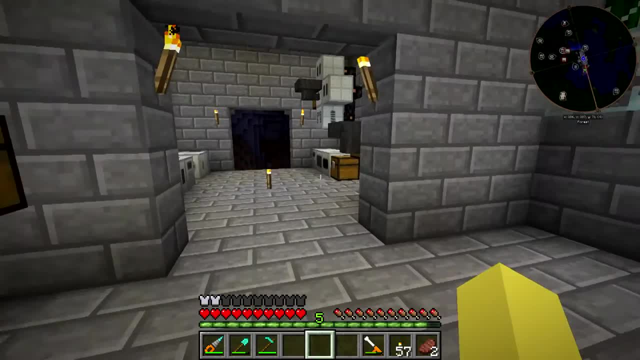 If you guys remember, I had some partially depleted ones from the old system when I put it in there, so I was able to get through those, but we still have 27 left. So before I do any crafting today, I'm going to bring these over here to the thermal centrifuge and start processing them. 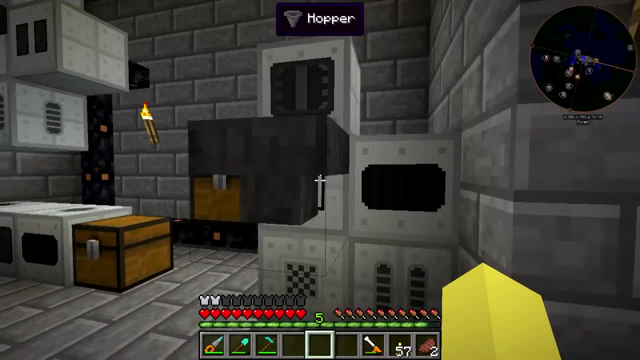 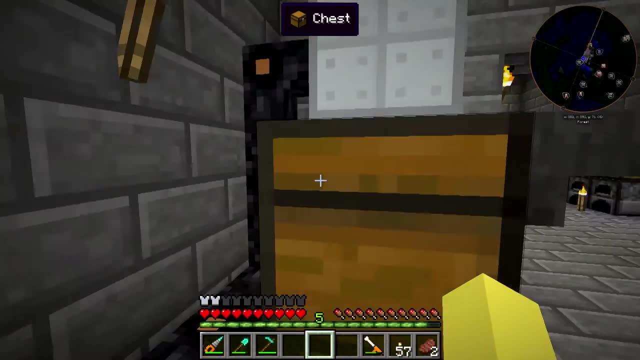 So I did want to show you guys what one batch will get us, and I still have a ton of uranium and stuff in here and iron dust, so we're not even going to have enough room in here to process this, but it'll just start filling up. I think it'll fill up the internal storage in here. yeah, it will. 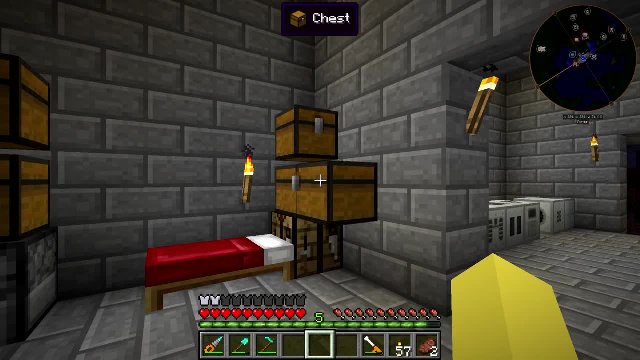 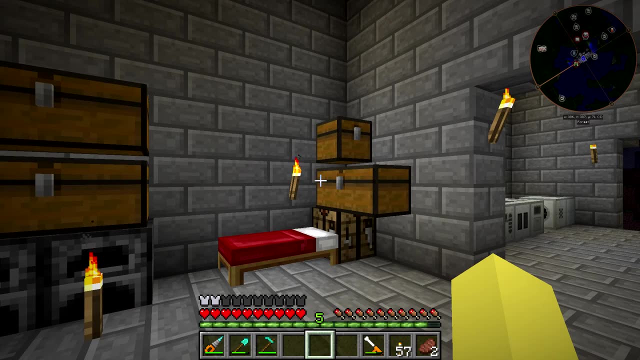 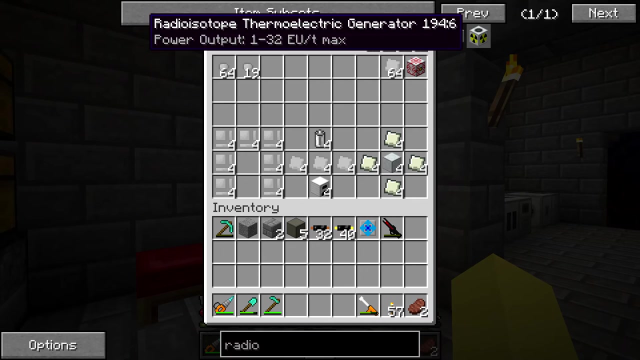 So we're going to start crafting, we're going to make these and then we're going to move up the whole UU Matter setup going on downstairs, which is the scanner, pattern storage, replicator and mass fabricator, and we're going to hook it up specifically just to the four radioisotope thermoelectric generators. 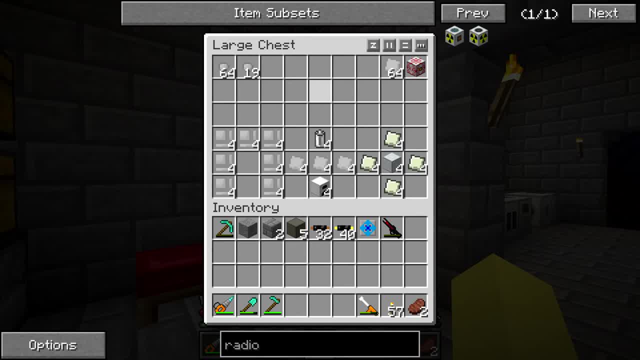 and I'm going to see how far I can push it. We're starting with four right now, but eventually we're going to move it to probably like as many as we can honestly get, which should exponentially scale as we get more power. but I'm rambling at this point. I got to jump into things. 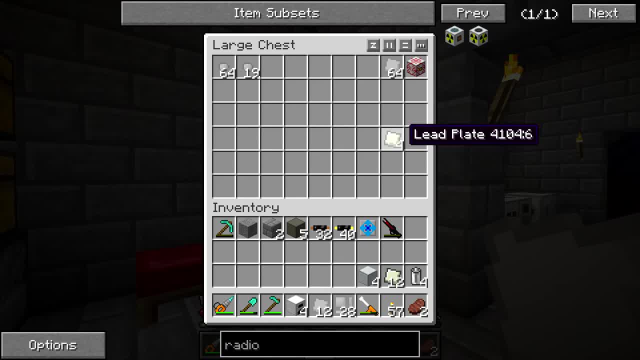 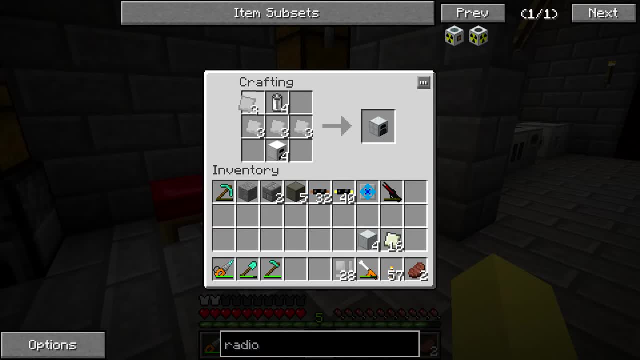 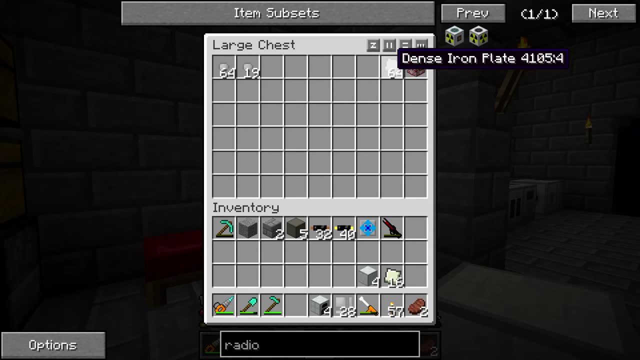 So grab all this stuff And start crafting. this is actually relatively inexpensive to make. it takes a ton of iron really. the most expensive part of this whole setup is just making the RTG pellets because they each take dense iron plate. that's not regular iron plate, which is nine regular iron plates. 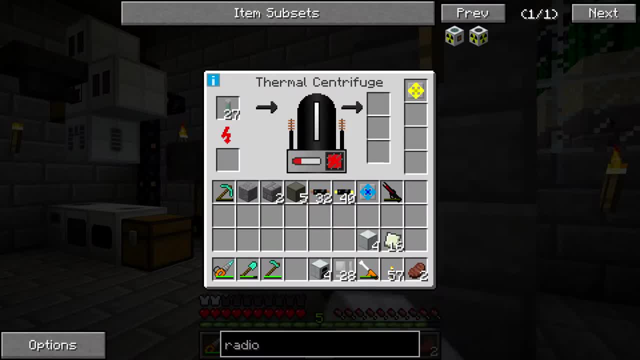 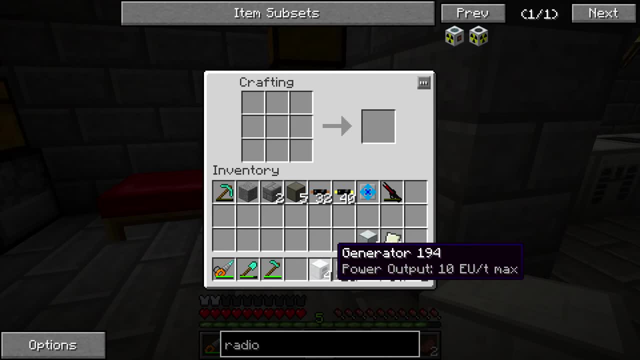 so that took a lot of stuff. Luckily, every time I process some of these depleted uranium we do get one thing of iron dust, so it does return a little bit. but eventually I have to use that to make more of the fuel rods, so it really doesn't give you anything, just kind of recycles it a little bit. 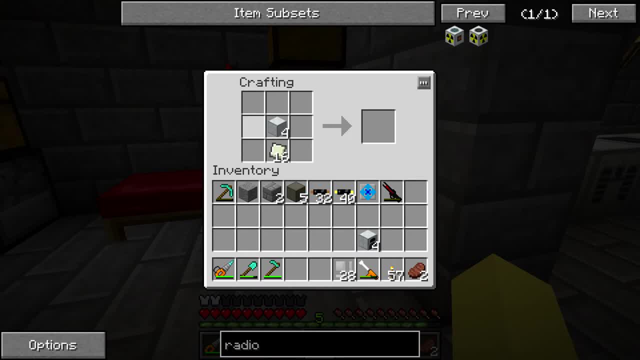 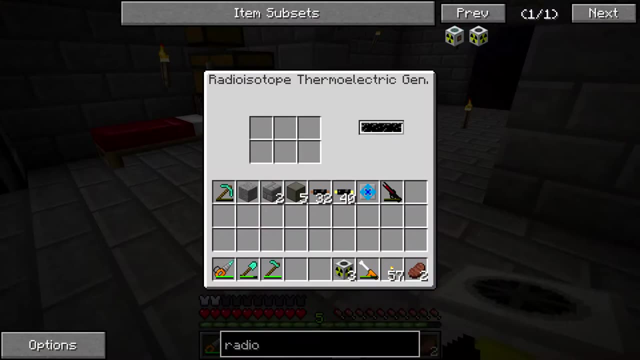 But now what we need to do is make the reactor chambers, which luckily, don't take dense lead plate, they just take regular ones. and lastly, we just got to surround it by the iron item casing. So there we go. we got this right here, same as the other one. I'll just throw it down to show you guys. 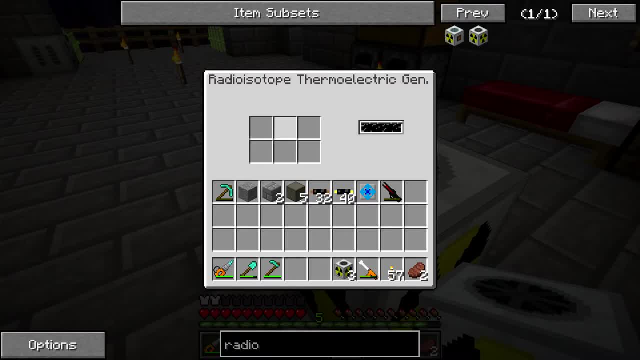 It looks pretty cool, but you can see that we've got the slots in here to fill in six RTG pellets. Now, if you haven't seen the previous video, I do want to explain how this works. So, essentially, you throw in an RTG pellet and that pellet is going to last forever. 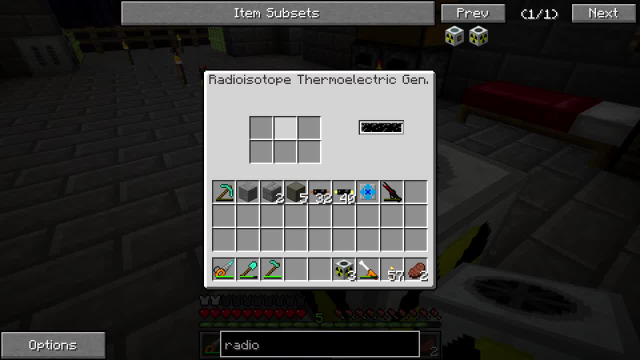 It's unlike, you know, other radioactive materials. it does not decay, doesn't have half-life or anything. it is just going to sit in there forever and generate power or, if you're using the heat one, generate heat based on being in there. 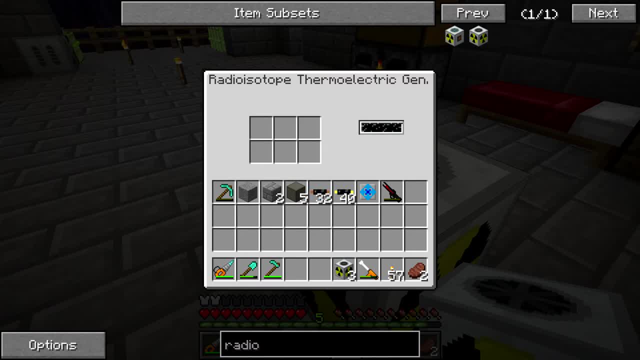 So it's essentially a better version of a solar panel and it goes up exponentially as you throw more and more pellets in there, between 2 and 64. Here it would have been 1.. Then I believe it would be 1,, 2,, huh, I don't even know how it would scale for this one up to 6.. 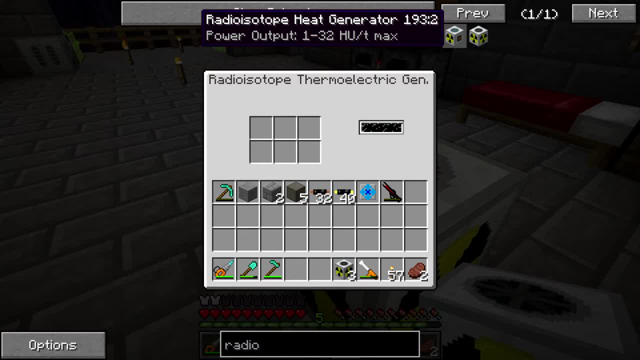 It would be like 1,, 2,, 4,, 6, or 8,, 16,, 32, I think would be what it was. yeah, So like multiply by 2 each time, but this one, it goes to the 2,, 4,, 8,, 16,, 32,, 64. 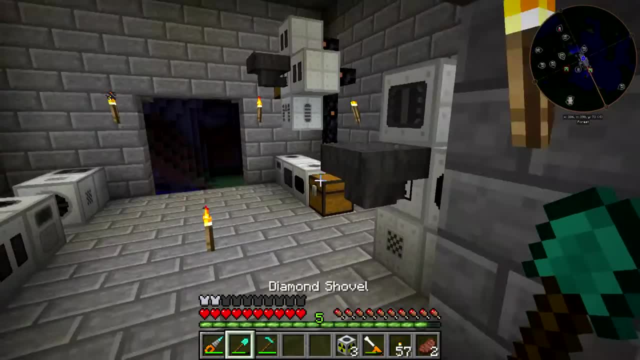 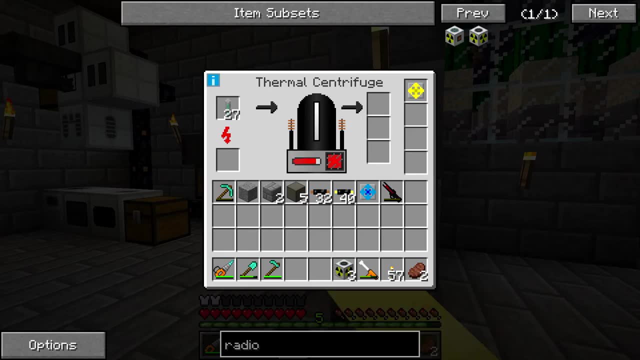 So pretty much just exponentially increasing by, you know 1. It's 2 raised to however many of these you have in here if you're curious. but these should start processing soon, so I'm kind of hesitant to craft these tiny piles of plutonium into plutonium. 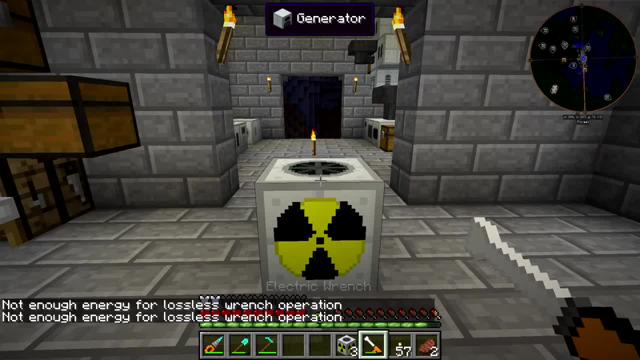 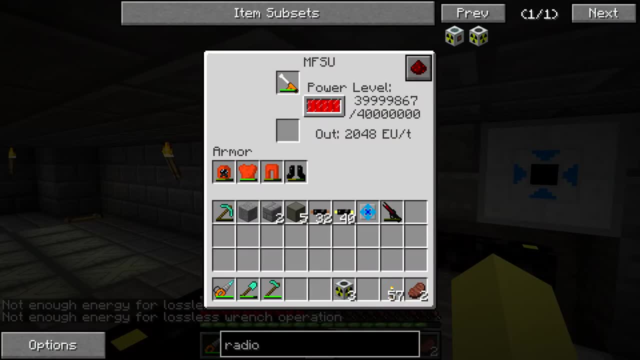 until we have all those done. so what we can do now is start moving this stuff over here. Not enough energy for lossless operation. oh my gosh, I really do need a backpack for these, or a bat-pack, whatever you want to call it. 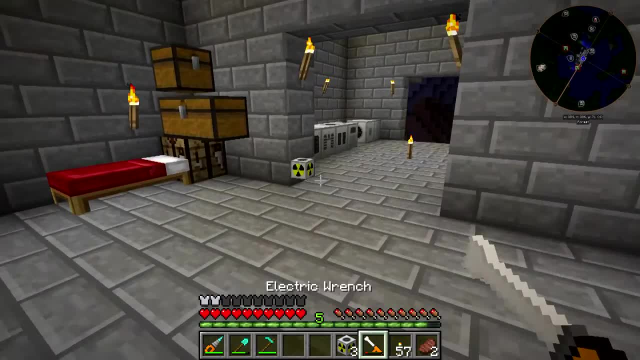 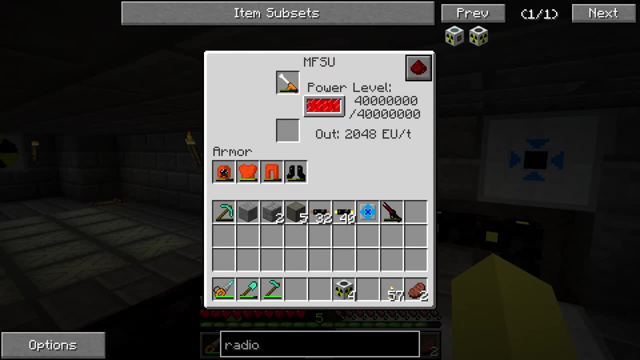 because I am going to use so much energy moving all this. so yeah, look at that, It's not really that much energy in the grand scheme of things, but the internal storage on this thing is horrific, so we can throw it in there, and then we got to grab all these things. 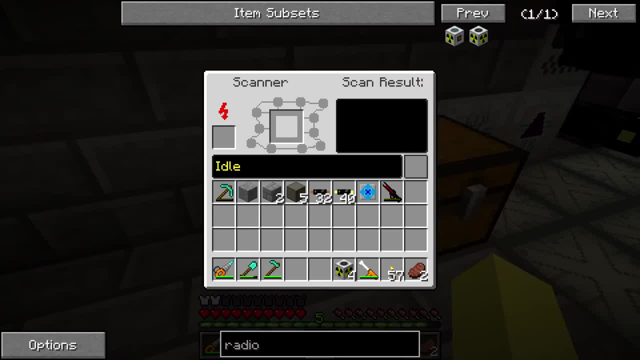 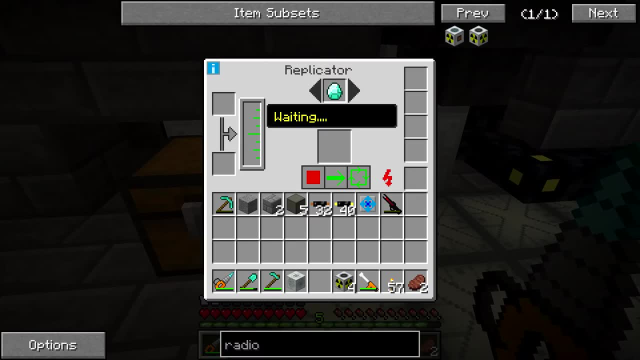 off the wall over here. So I don't know if these lose what they have in them. so obviously the scanner's got nothing in it. right now We can pop that off, but right here the replicator, I do. yeah, there's actually nothing in there. 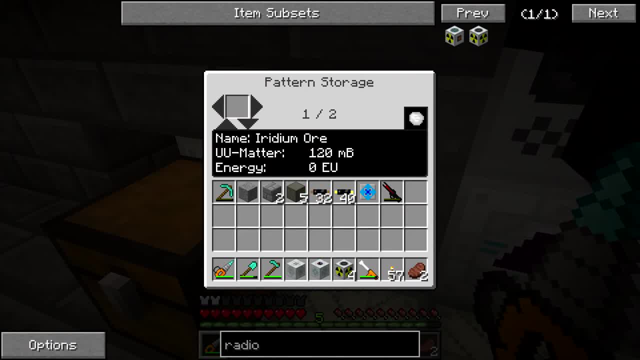 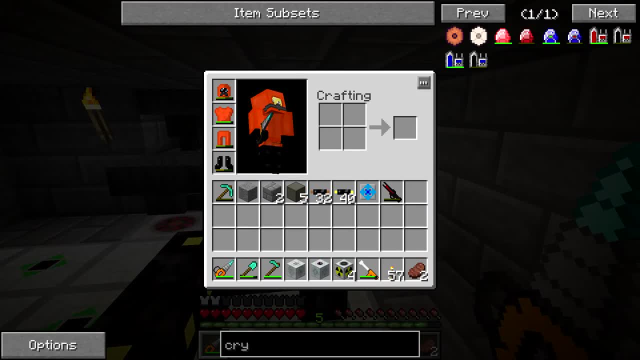 It takes the pattern from the pattern storage, so we get that off. and I'm pretty sure here if I wanted to do, we want to go make a crystal. Do I have what we need to make a crystal right now? Uh, I do not. 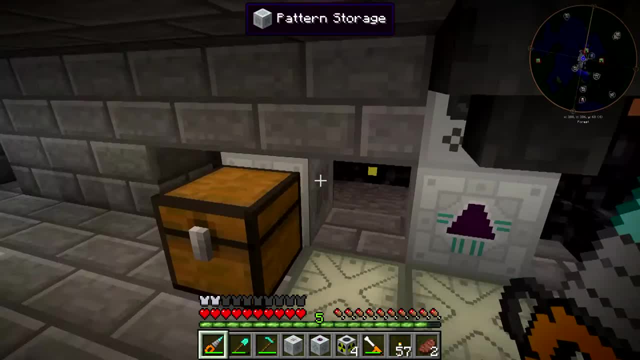 I don't have obsidian dust right now. Okay, so if this loses what it scanned, it's a little unfortunate, but we can rescan and stuff. I suspect it does, and that's why you'd export it to a crystal before you move it. but we're 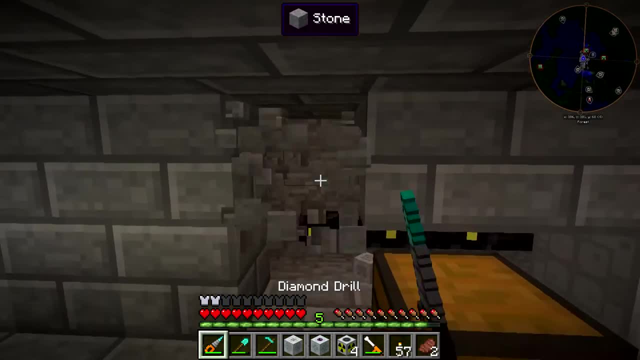 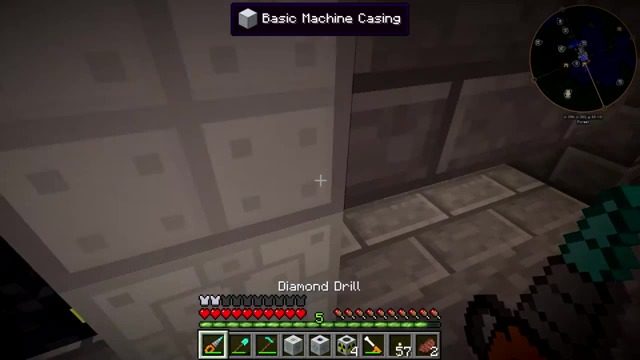 going to grab this and come on, let me get back there. I finally am using the drill. I've used it before when we're making the reinforced stone, but that's really it. so now I'm finally using it, because this is pretty much dead. 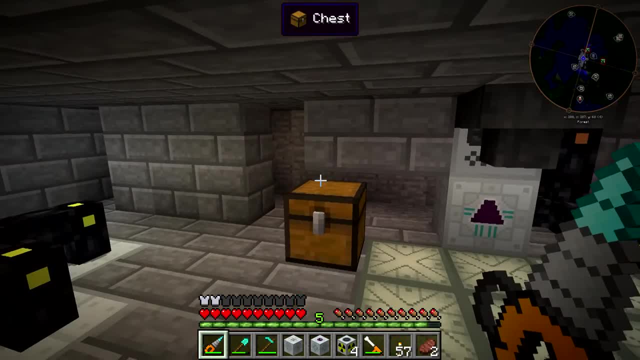 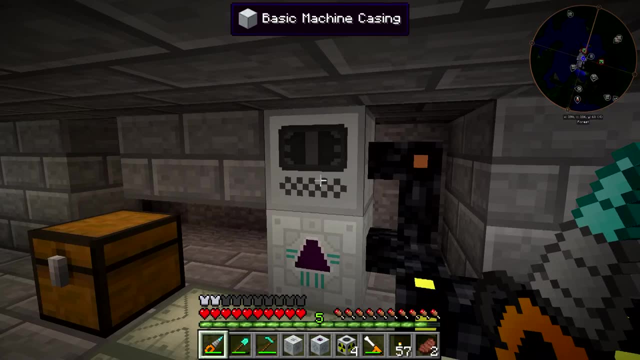 I might as well just throw this out, but huh, we're going to have to cover up that wall and now we can break this, and yeah, so we just have the recycler here, Grab this out and where's my wrench? 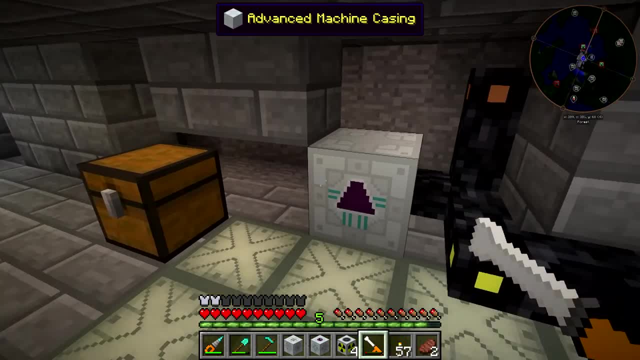 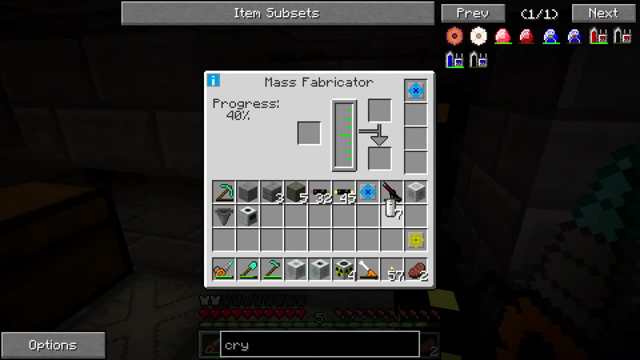 My wrench is right here, So I'm going to try and do a better job of maintaining using the recycler, as it pretty much makes it roughly one-tenth of the energy cost to make one millibucket. but we can grab this out and oh you know what. 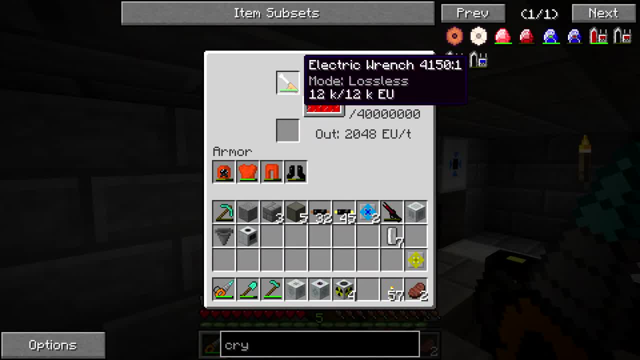 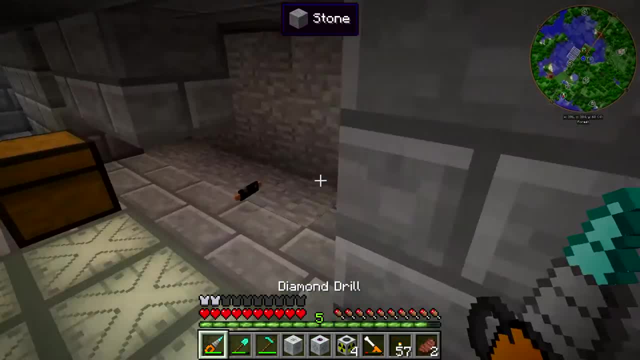 We're going to need to refill this. Okay, there we go and grab this. Okay, so we can also just get rid of all these. and now there's not really going to be anywhere for this power to go at the moment. 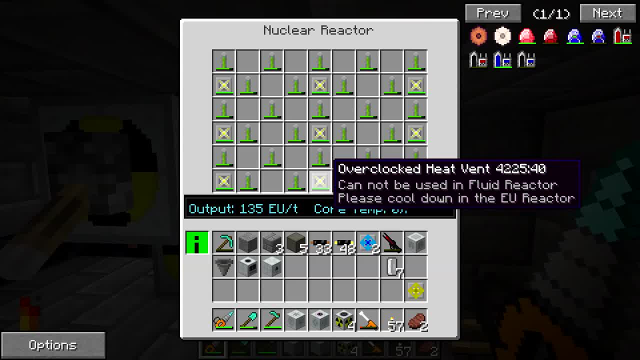 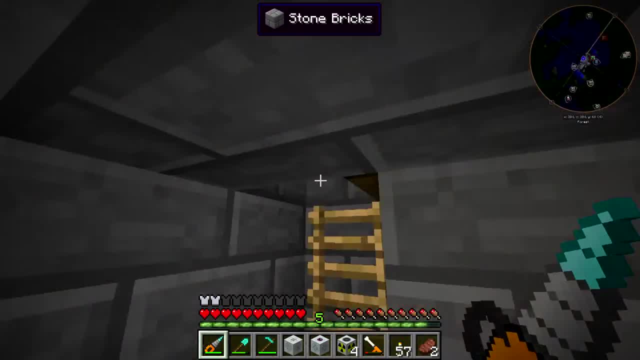 But I can just hook it up over here and then I really don't care about the energy coming from this. This is a whole new batch of uranium that's sitting in here, so you know this will be processing while we're setting all this up, and you know that should lead to another. 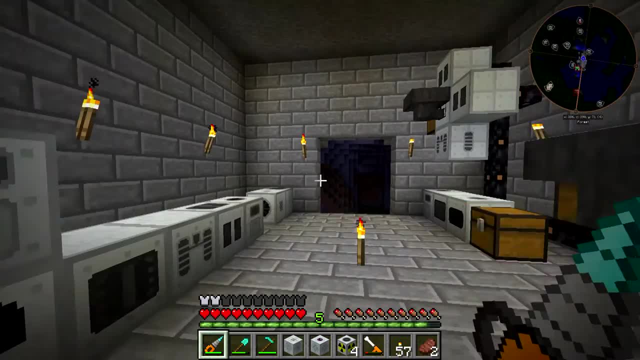 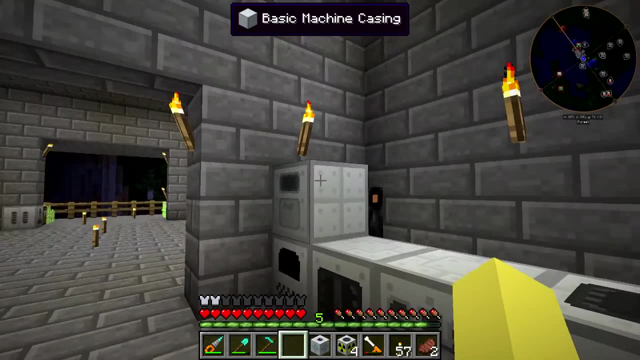 that would be each one of those. I'm actually not sure how much that would lead to. I don't know the exact number of plutonium that you get from each or tiny pile of plutonium, I should say from each of the fuel rods. but we can make a little bit more because 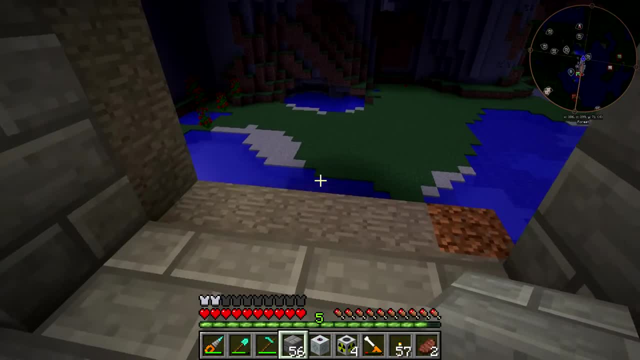 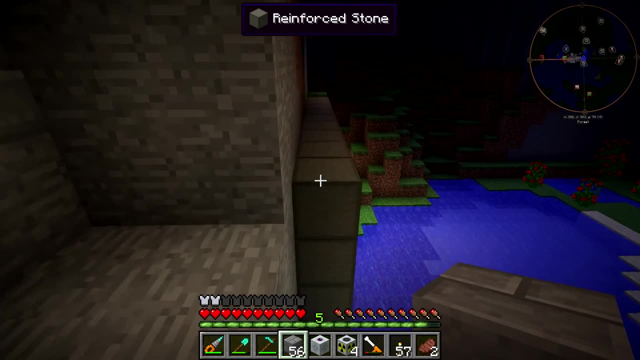 we're going to be making the room right over here. Obviously, that's why there's a hole in the wall. I just decided, eventually, that we're going to be building out here. No one's going to see it, but us. So after I made the reinforced stone out here, I thought: you know what? 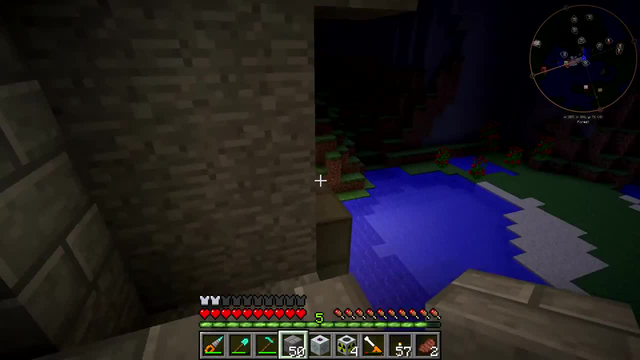 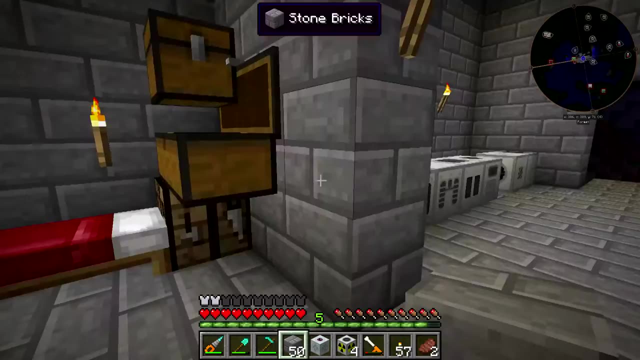 Screw it, Let's just- let's put rooms off the back over here so I don't have to worry about expanding, and eventually maybe I'll just terraform out there and cover the whole thing up with stone, Who knows? But is this? oh man, that's not going to be close to being done for a while, so maybe 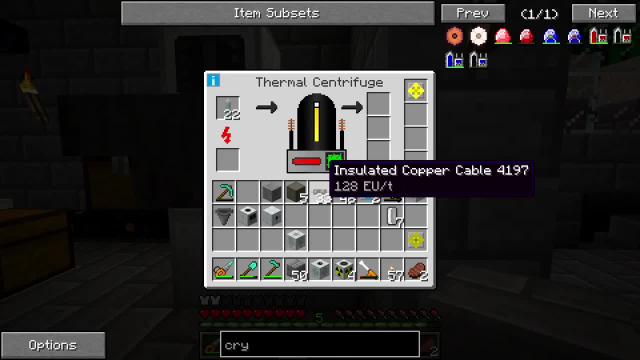 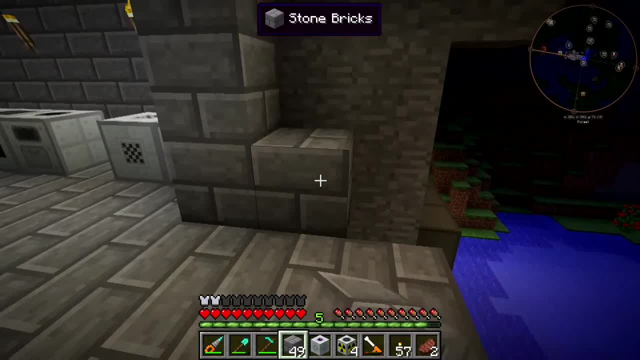 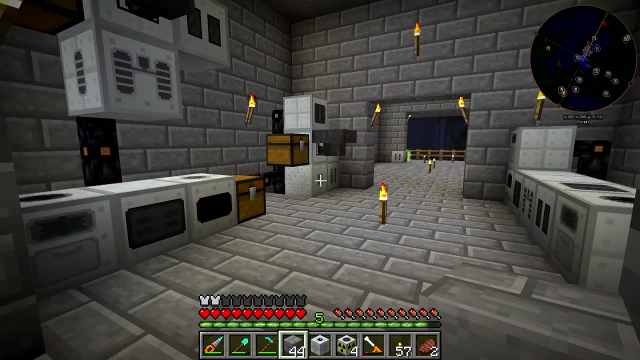 we won't use these tiny piles of plutonium- Plutonium on camera, but whatever. Luckily, when I processed the ones that are sitting in there, the tiny piles of plutonium, I was able to process the extra dual fuel rods that I had because I cycled through on. 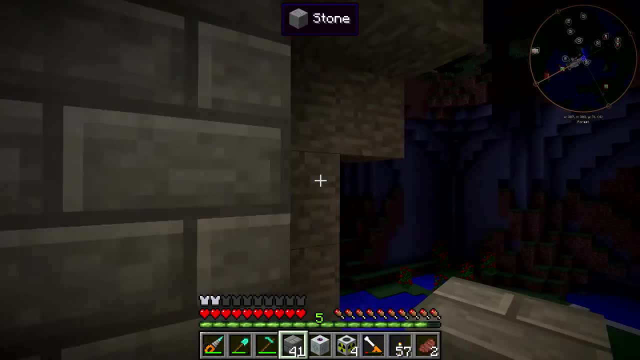 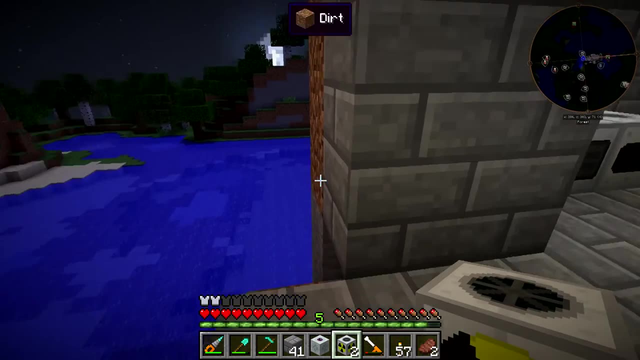 the liquid nuclear reactor, which actually uses the dual fuel rods. so it got me a little bit more, But what I'm thinking we do is just put these on the wall and then we can wire them. So throw them like this And if you're wondering, 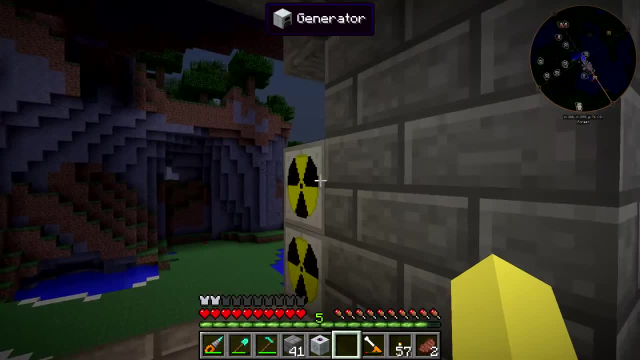 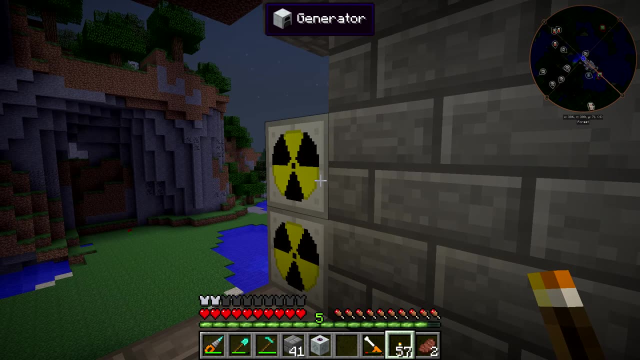 what you should do to set these up. you should fill one up at a time because, since it goes up by multiples of two, if you were to use four and one, then you would be getting what? 16?? But if you were to get four spaced out, you'd be doing two, two, two and two. 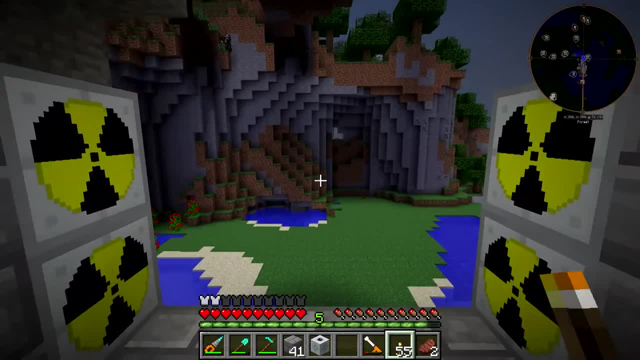 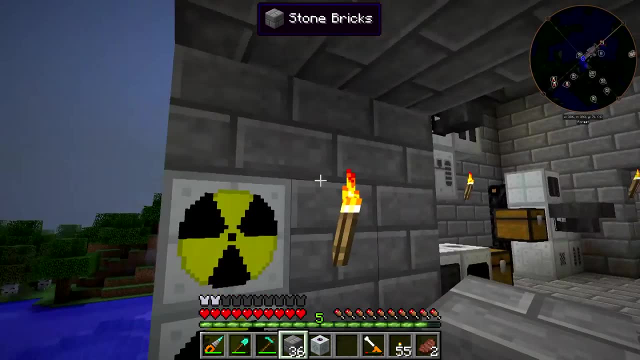 So you'd only get eight because it's not multiplicative. So multiplicative is better than additive in all the cases here. So I am going to fill in right here, but eventually I'll put like another one up there and maybe even put them right here. 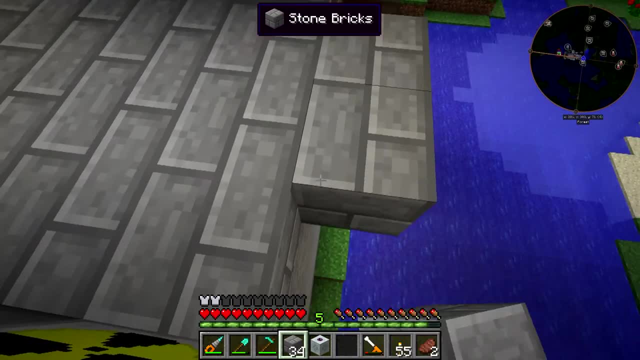 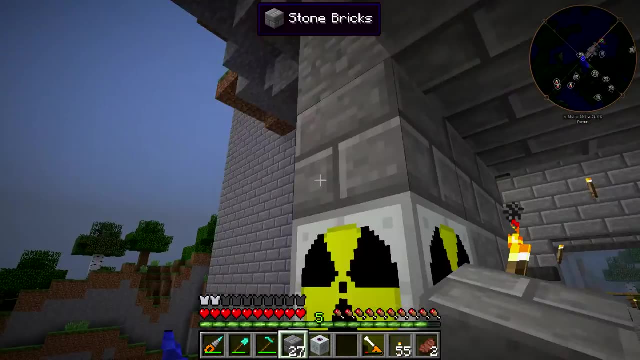 I do want to keep it doorway, But got to expand this out a little bit more so that we can start throwing down the replicator stuff which should probably will go one one more back, just to leave some room. It'll take forever for me to fill these up, actually. 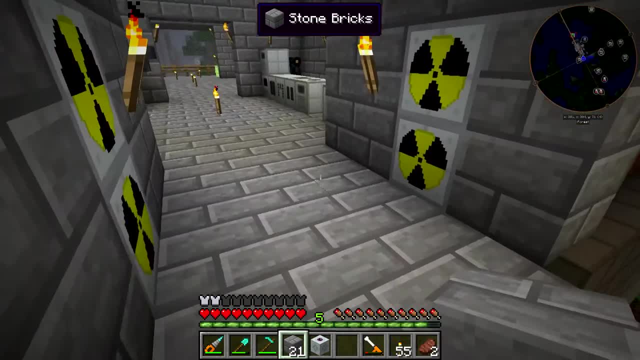 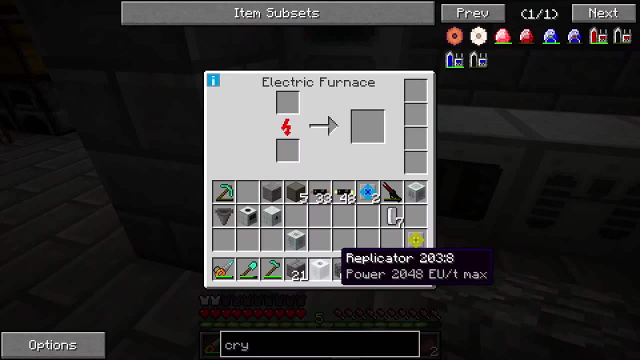 So I'm not super worried about expanding, but we'll build right here And I should actually probably get cooking down some more stone. Got a lot of cobble in here. That's really all I use the chest for now is just storing cobble. 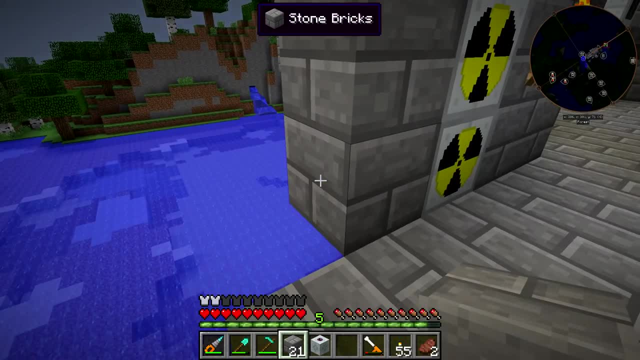 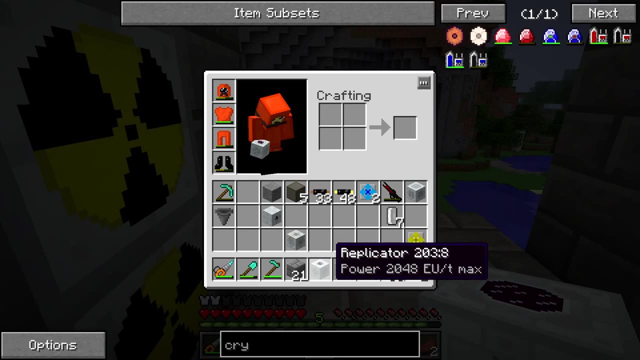 But okay, so we come over here and I want to throw these down. Try to think of the best way to throw them down, Because we want them to be able to send things to one another. So I'm thinking we want the scanner. 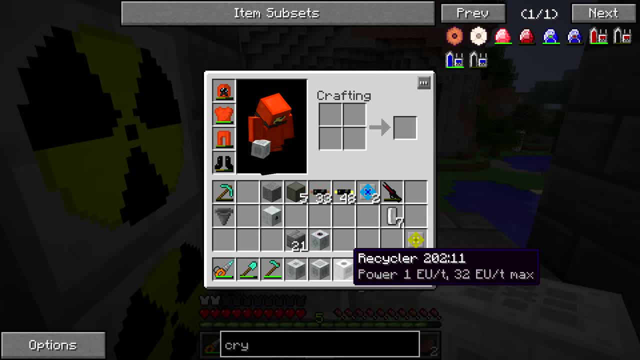 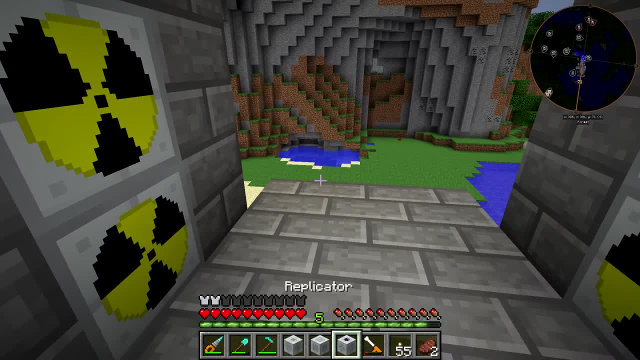 The scanner needs to be next to the pattern storage and the pattern storage needs to be next to the replicator is what it is, So these need to be next to each other and the replicator needs to be able to get things. So I think we can just do them across the bottom here. 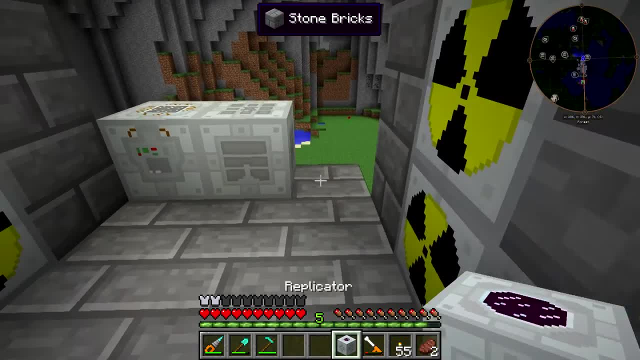 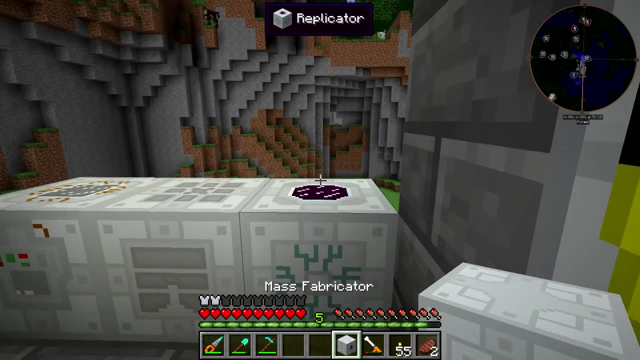 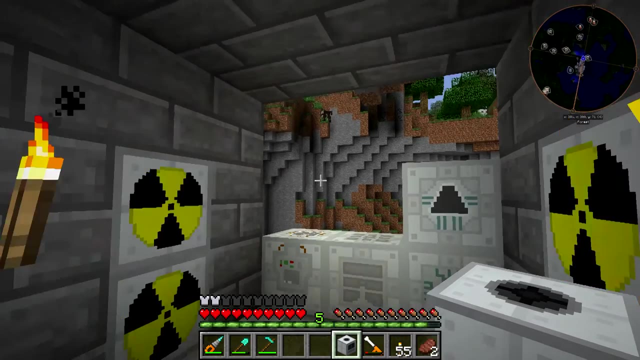 I think, right, so scanner pattern storage replicator like that, and then we're going to have the mass fabricator right above it, right over here, and we can have the recycler. all man, This looks so weird, This looks so weird. We can have the recycler like right up here, right? 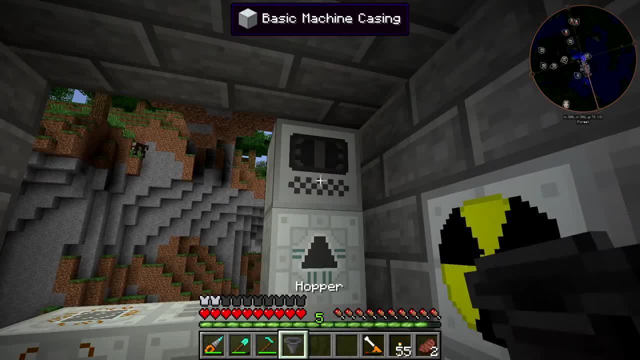 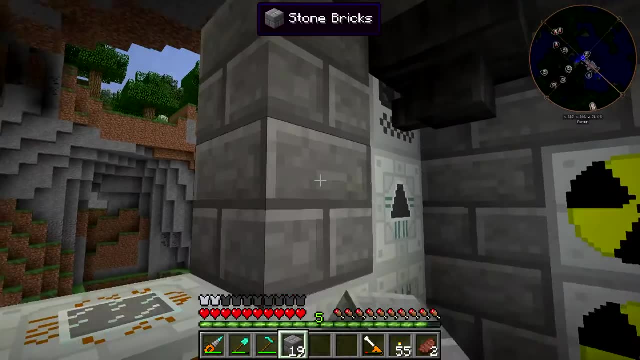 Yeah, we just put that up there and then I can just throw the hopper down right like that. That looks really bad, but whatever, fill it in. So I guess we actually didn't need more stone. We actually shouldn't fill it in completely yet, because we do need to. 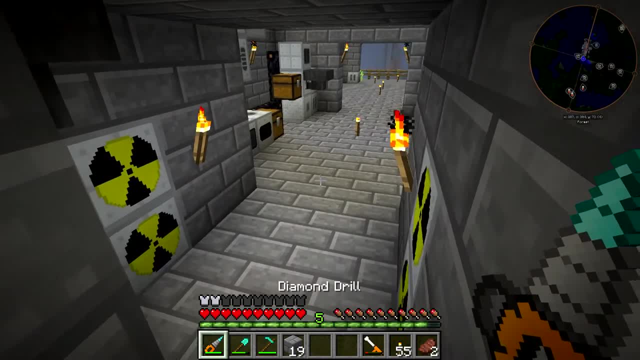 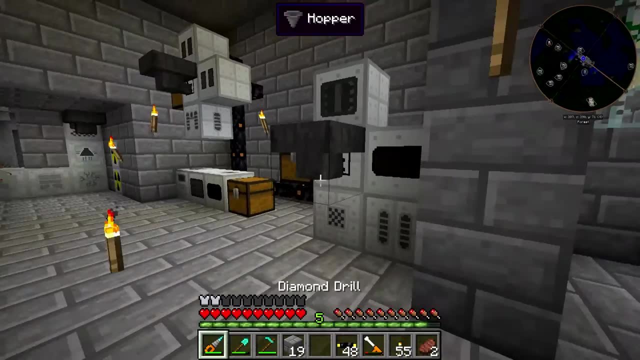 Wire power from these, so each one, assuming it's at its maximum output, should be fine with gold cable for now. So I actually have that on me. Cool, How is this going? Okay, so it's at 15.. It's getting a little bit extra. that should get us being able that. that'll be three. 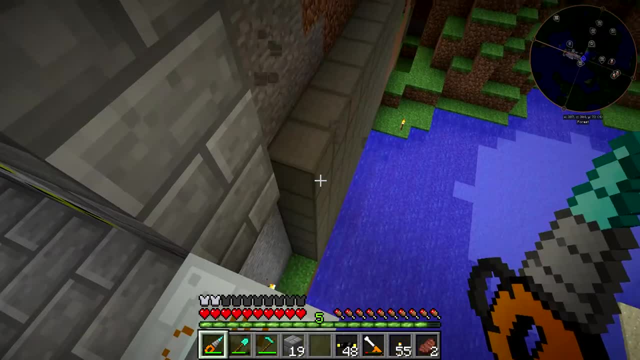 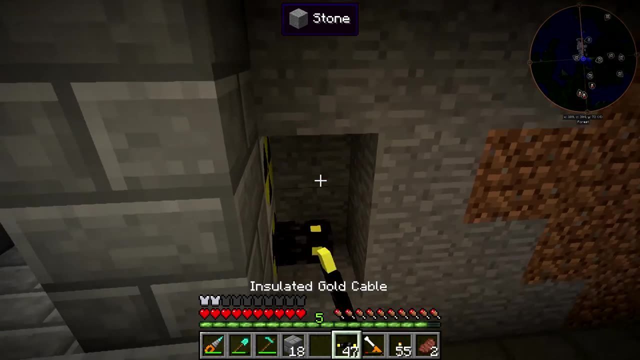 So that'll be one pellet. That'll be one extra pellet that we can use. so break that and I'll just put this here. So it's a little bit easier to walk. but we're going to wire it from the back like so, and I want to. 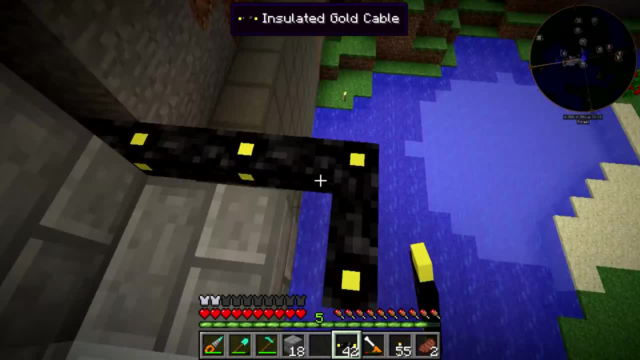 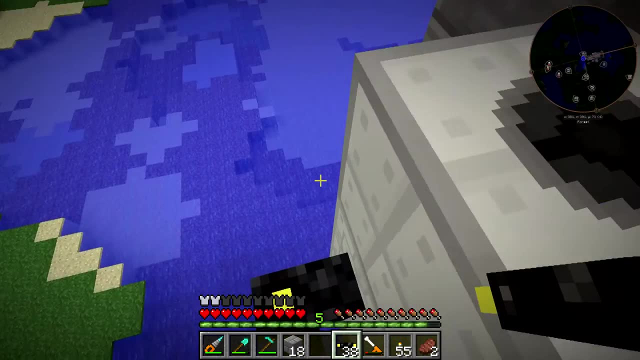 wire It like this, because I want to keep it on the same level down here as all of these machines, because we do need to wire both of these in there, and then we can wire this in, and then we can circle around and do the same thing over here. 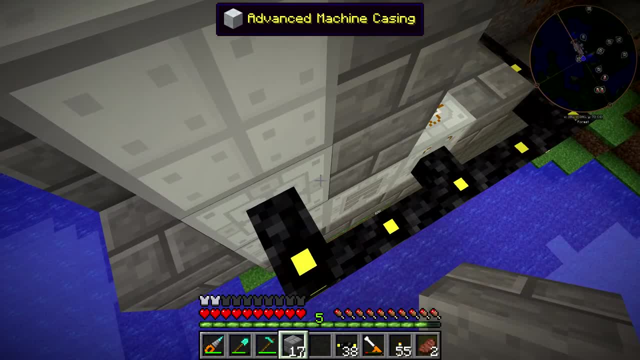 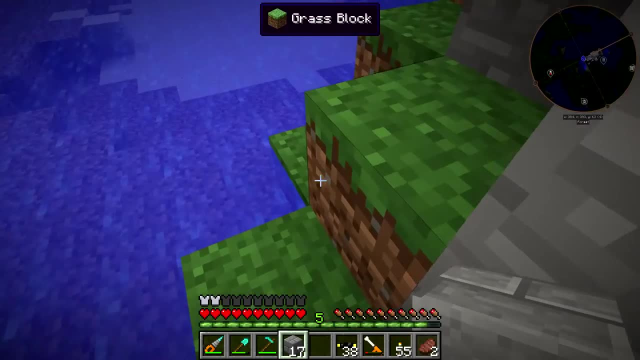 I'm going to put that the same like that: Yeah, it is, So that's in the set. Oh, no, darn it Huh. Do I pillar up? I don't think I do. I think I got to run around guys. 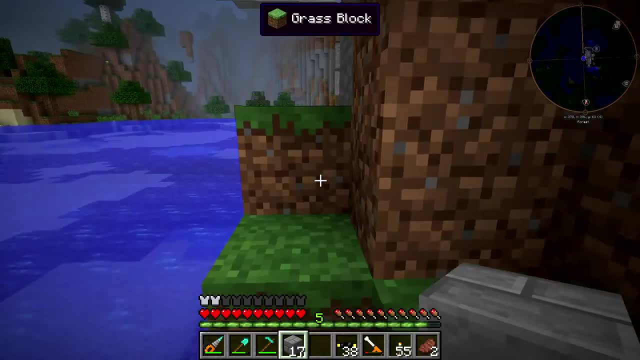 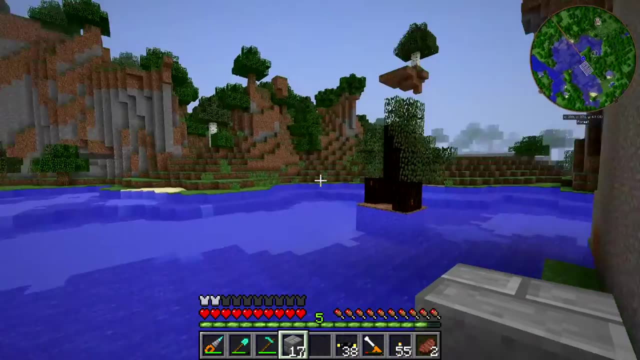 You're going to see why I should not be using I don't know It's. it's a conflicting Opinion of mine, because I don't want to get radiation, but I also want the ability to fly. I just don't feel like keeping my- oh gosh, my quantum armor in my inventory all the time. 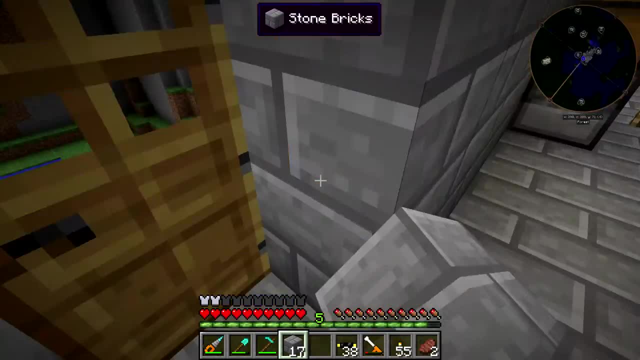 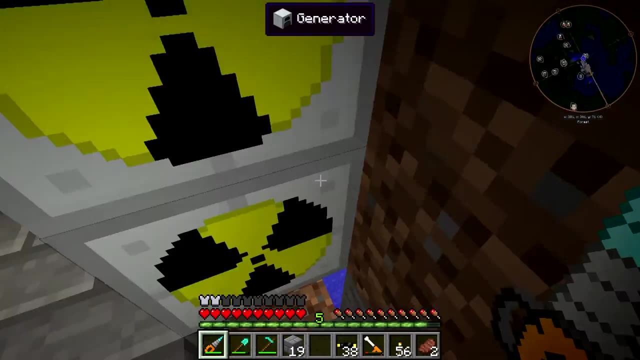 So it's really you know, it's just it's rough trying to decide: Okay, so now we just got to wire these around and then this will actually be okay to run. So I should just break this wall and we can wire them through here. 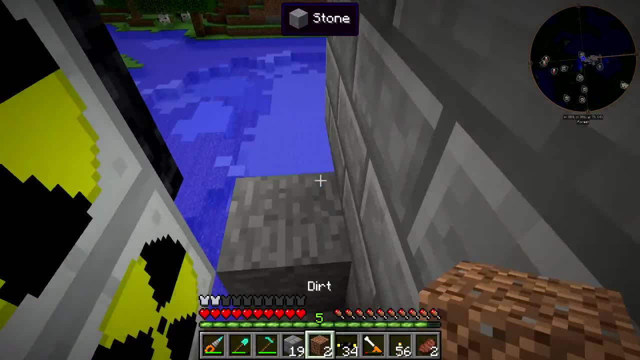 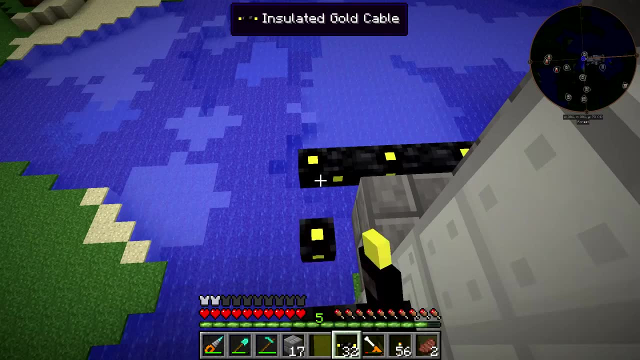 It's be a little bit easier. Wire it like this: fill this in right here, There we go, and come back out here and just connect the wires, There we go, And that's there is a stepping stone. If I need it, I guess probably won't need it. 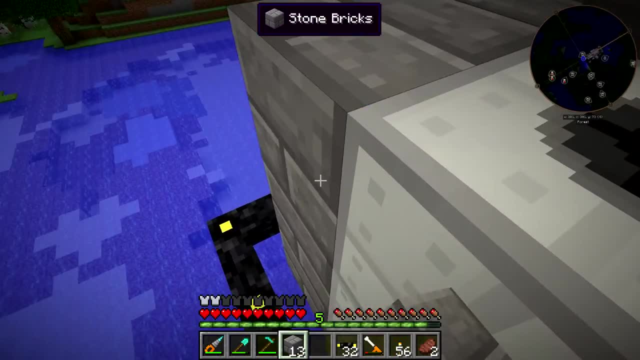 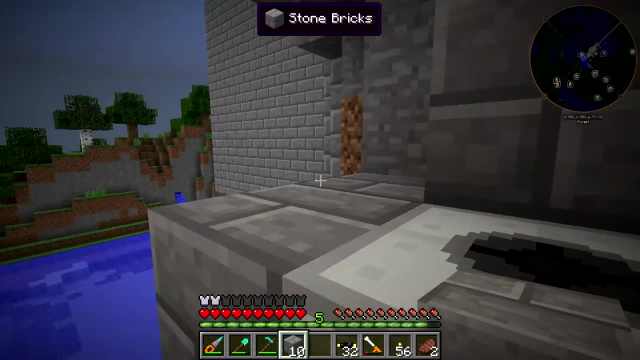 But I didn't even put that there. I feel like I'm just wasting stone brick. but let's just we'll cover this up. We'll make it look a little bit better out here And then we can cover up the top, because why not? 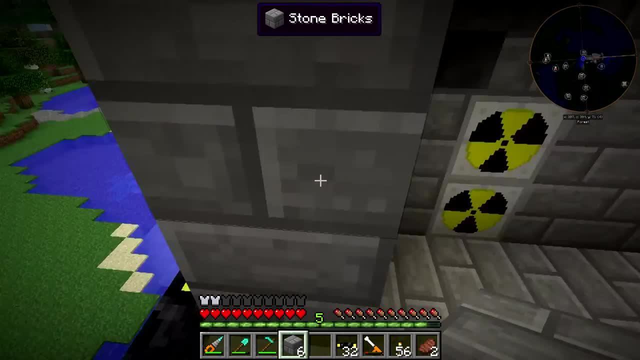 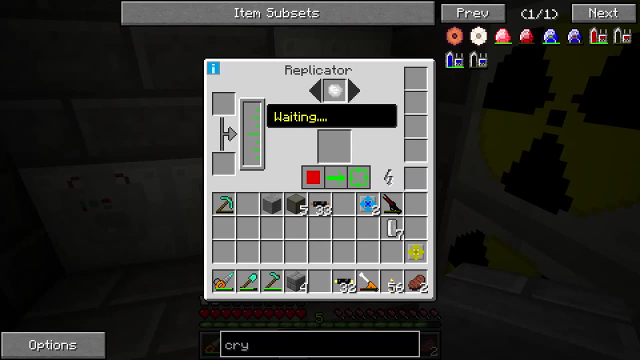 Oh my gosh, I'm throwing bricks everywhere, Throwing them everywhere. Okay, So there we go. That should be good. Did this lose? Oh, it didn't lose the patterns. Nice, That's awesome. Okay, So this did lose. obviously, what's in it? 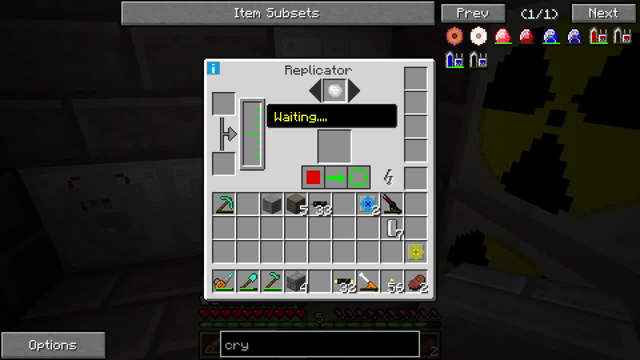 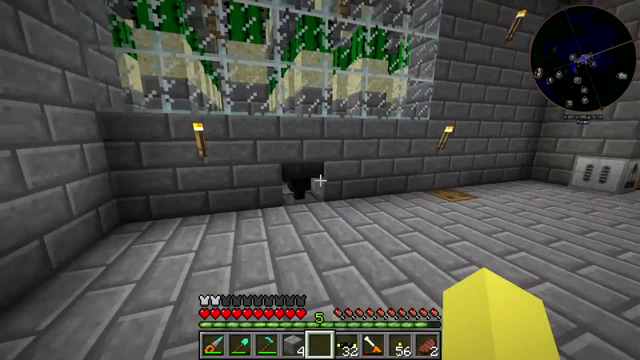 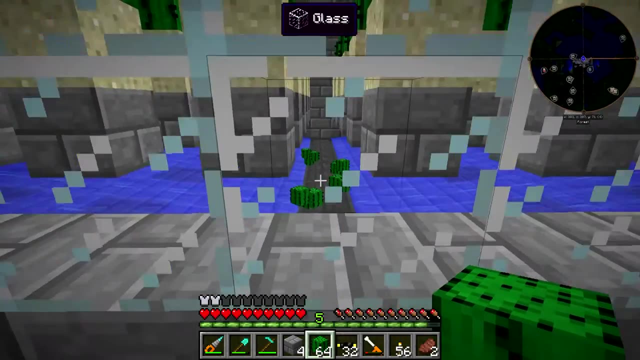 We did lose like 80 millibuckets, which is a little bit unfortunate, but it happens. and this is at zero because there's nothing running here and there's nothing in the hopper. So what we can do is start things out by getting a bunch of cactus here, and I should really make a better system for getting his cactus over there, because, as you can see, we have way too much cactus even with the upgraded system downstairs running faster than before. 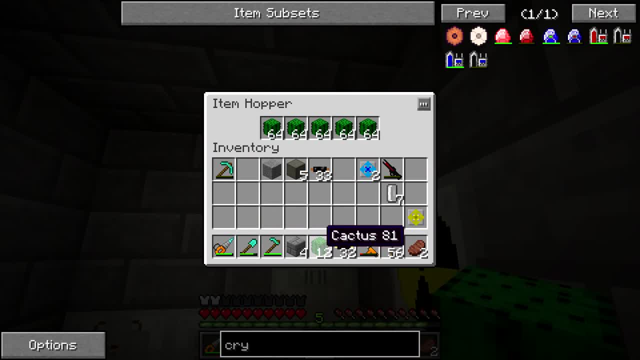 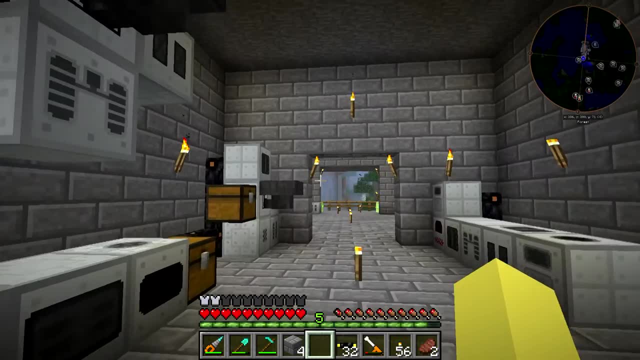 But I can use this with the recycler. It's phenomenal and I just need to get a better way to wire them over here, essentially other than just hoppers, but most of the time I manually transport it, So for the most part these should be okay. 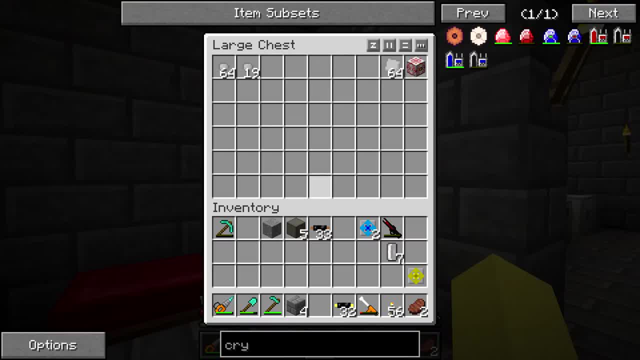 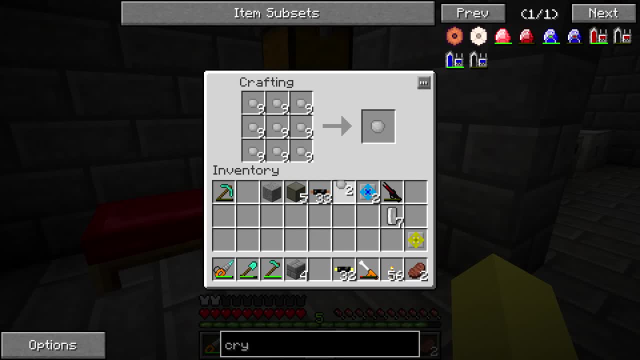 I thought that looked a little bit weird. We can leave that there. That's only one pellet, So we can come over here, grab the plutonium, start crafting this, and it looks like we're one short off another piece of plutonium, but we're at nine right now. 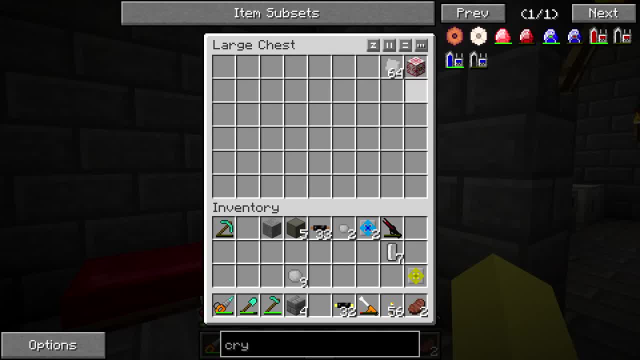 So that is great. That means that we're going to be able to craft three pellets, and does not what we want. I crafted 64 of these dense iron plates just because I wasn't sure how many I was going to be able to make. 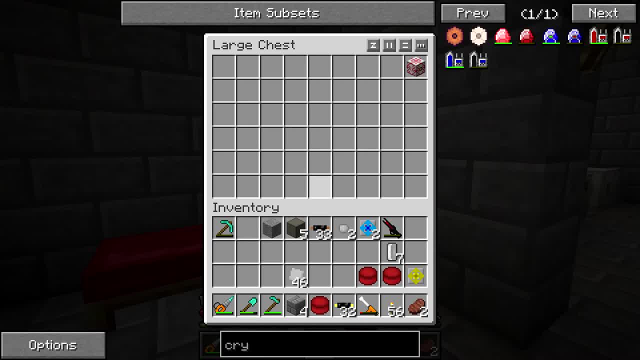 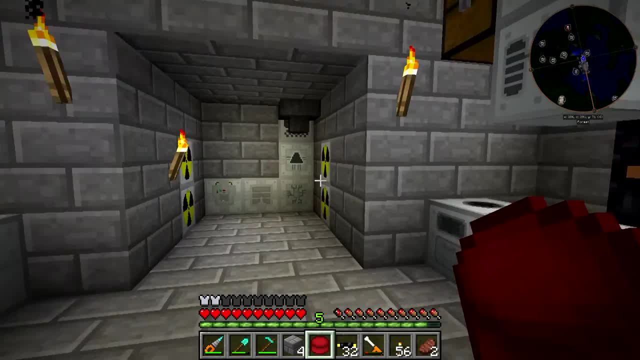 Unfortunately, we're not going to be able to make that many, So luckily for me, that means that while I'm working on this, I don't have to worry about these dense iron plates and crafting more of them. I can just, you know, use those as we go. 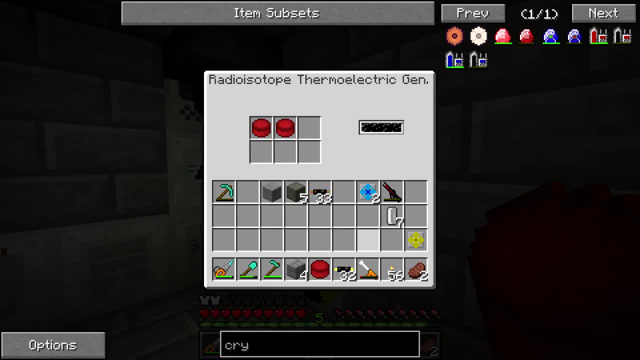 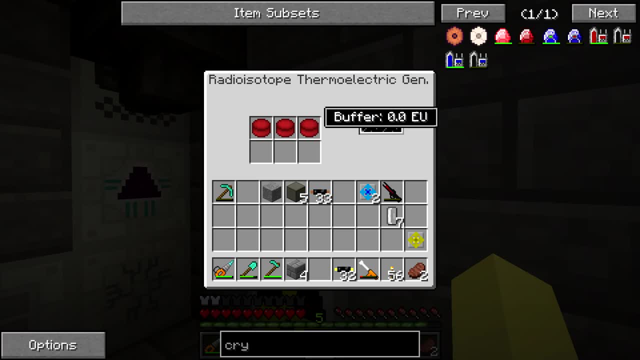 It took me forever to get that iron, but we can throw these in here and it should start generating power. You can see that this thing kicks on now. It doesn't tell you how much It's actually generating, but I believe the heat one does. 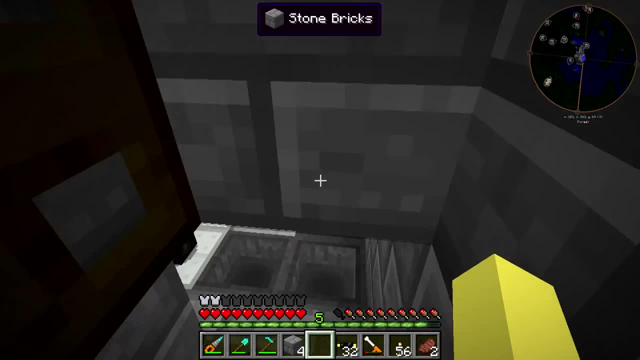 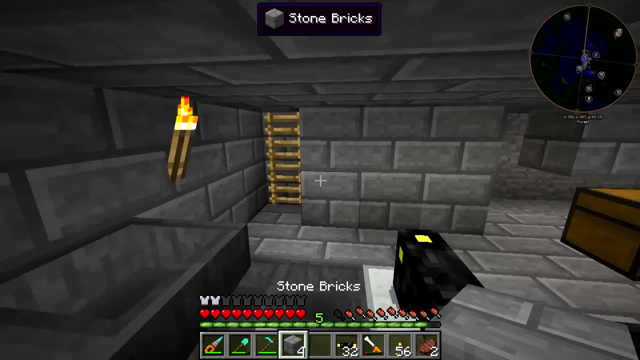 So let's go. I want curious. I want to see this. I think the heat one tells you how much it's generating at the time. So we do have to come down here. Yes, This one tells you, the other one doesn't. that's weird. 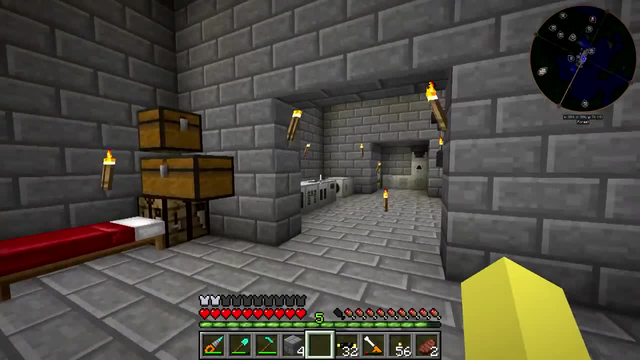 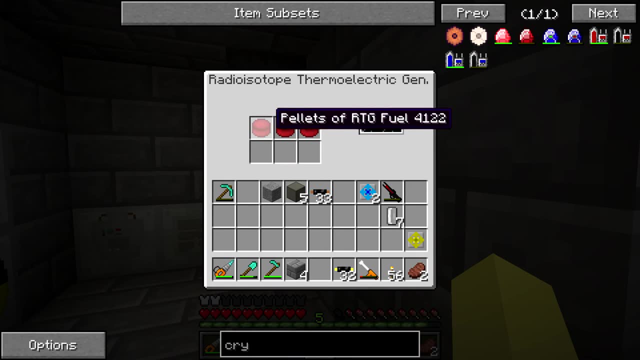 But assuming they work the same way- and I'd be interested to see this- one should be getting right now eight EU per tick, which is that should be eight, right? Yeah, two, four, eight, So nothing fancy. This is going to go really, really slow. 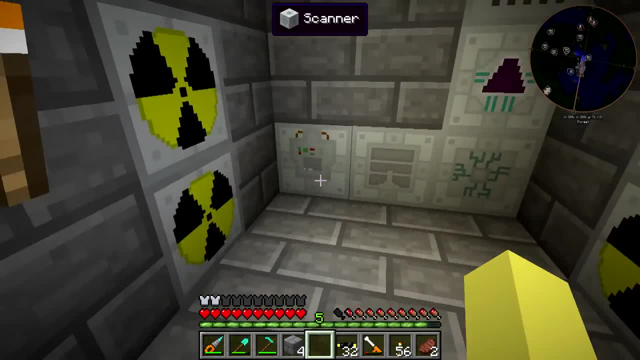 And not to mention the recyclers going to be run on the same power for all of this, and pretty much everything is going to be filling up right now. So this is filling up, Everything's filling up. It's not going to get almost any energy. 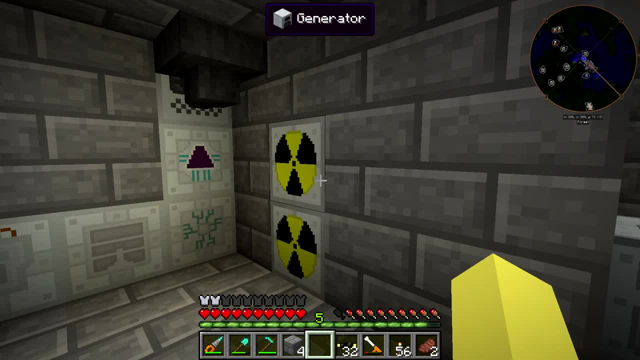 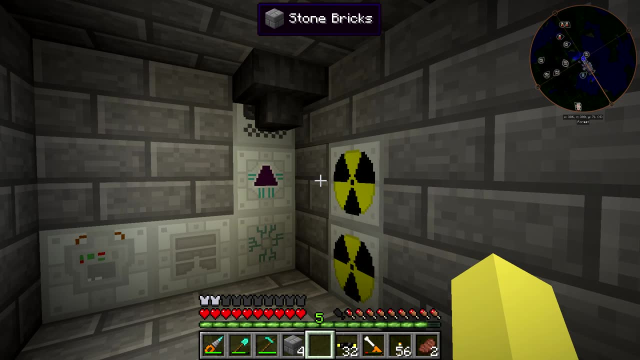 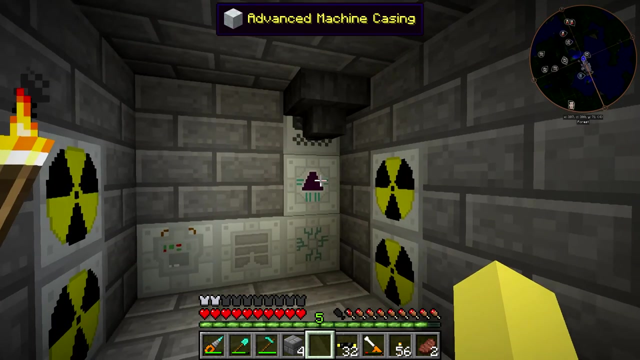 But once I get all of these full- getting 64, I think it'll be a worthwhile project, think it'll be pretty cool because I have so many things around my base right now- They can explode, kill me, destroy everything, ruin my life- that it's nice to have something that I can just leave and not have to monitor, not have to worry about it blowing up, not have to worry about any of that. 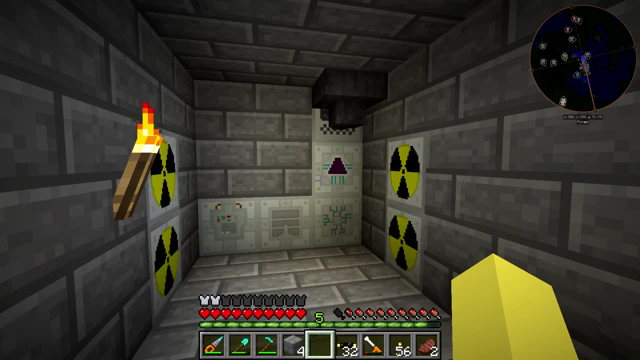 It is Very, you know, different than what I normally have, and I just think it'll be a fun project. So maybe every couple episodes I'll jump back here See how things are doing, pretty much just, you know, every two hours and 45 minutes. 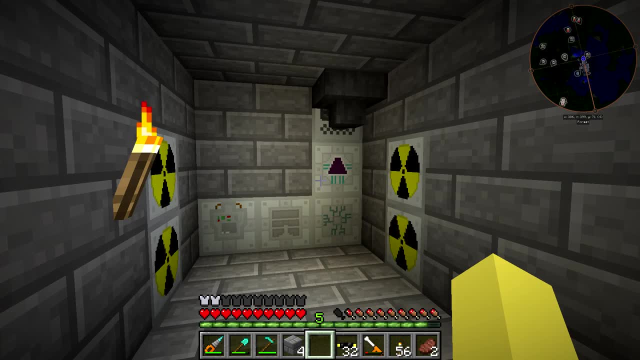 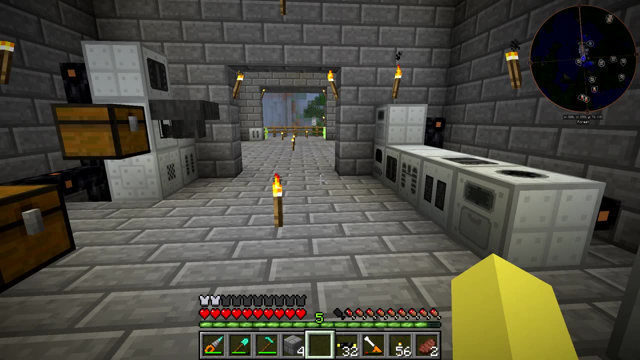 I spend in the game I can probably make. the one reactor that we have going downstairs That's specifically for plutonium is going to be able to get me one pellet per three hours in game. Then we have the mox reactor, which we're going to pretty much used to refill itself. 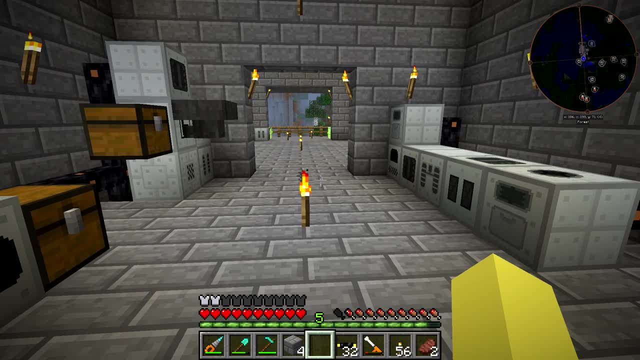 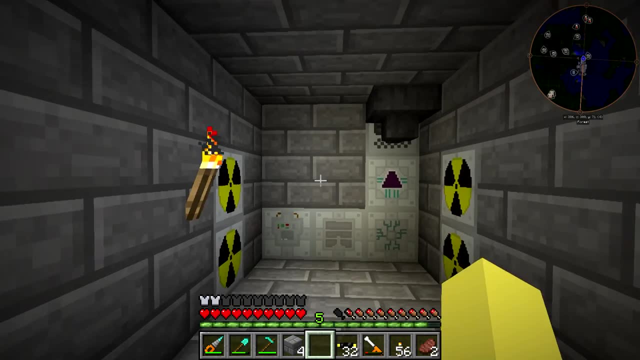 So that'll get us nothing. And then the liquid Cooled one is going to be used to at one point help maintain the mox reactor, and then after that all the extra will come up here. So it's probably like roughly two pellets every three hours.